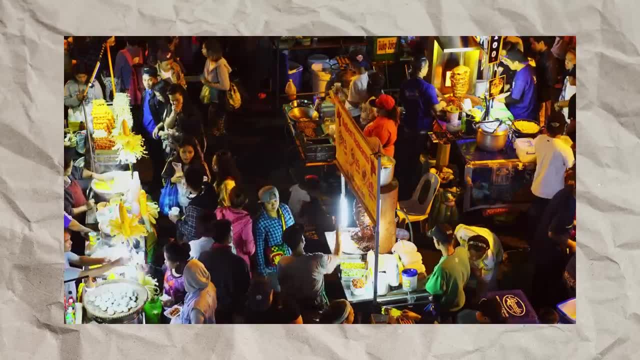 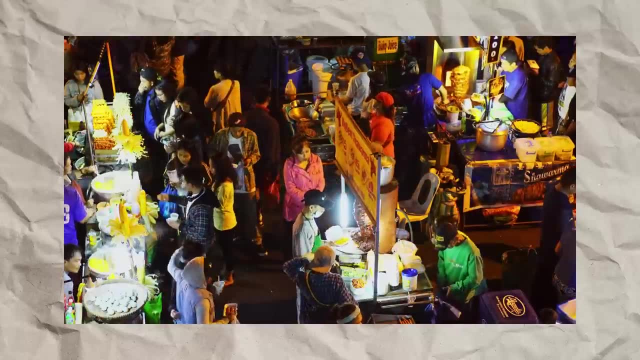 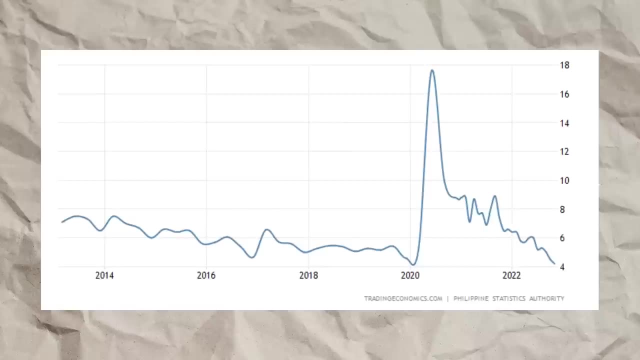 Another important factor in the Philippines' growth was the country's high employment rate, which pushed up consumption despite inflation. According to the Philippine Statistics Authority, the unemployment rate dropped drastically from 6.4 percent at the beginning of the year to less than 4.2 percent by November, the lowest rate since 2005.. The National Economic Development. 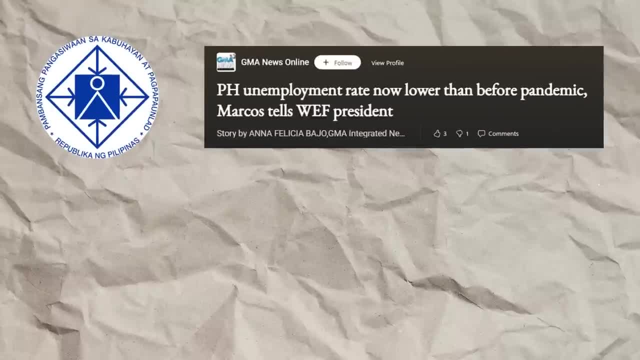 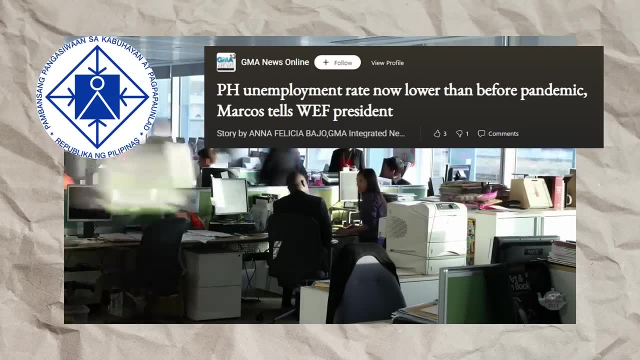 Authority said, attributed this drop in unemployment to workers finding more renumerative and stable work in private establishments, as well as an increase in full-time employment. While services were a strong contributor to the country's growth, there were also sectors that didn't fare as well. 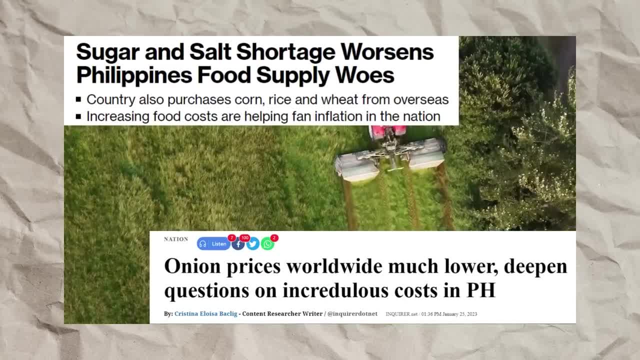 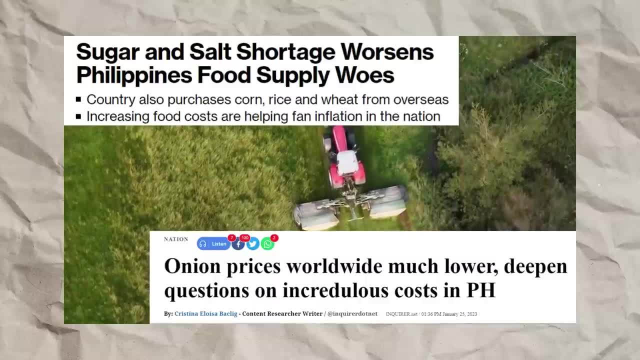 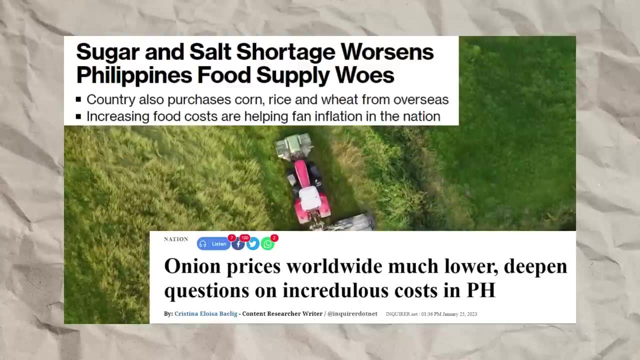 The agriculture, fisheries and forest industry, for example, saw a decline of 0.3 percent in the fourth quarter. Economists have noted that 2022 was a difficult year for the agribusiness sector due to an increase in natural disasters. The government has continued to support consumer. 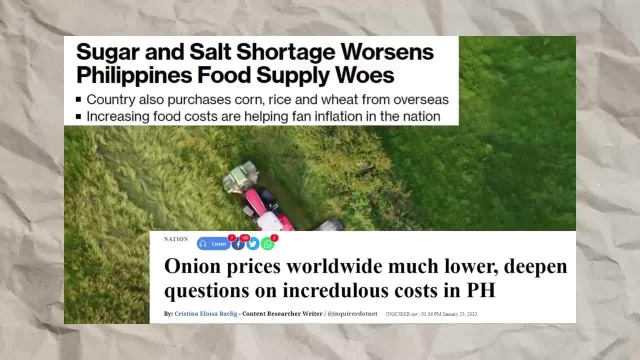 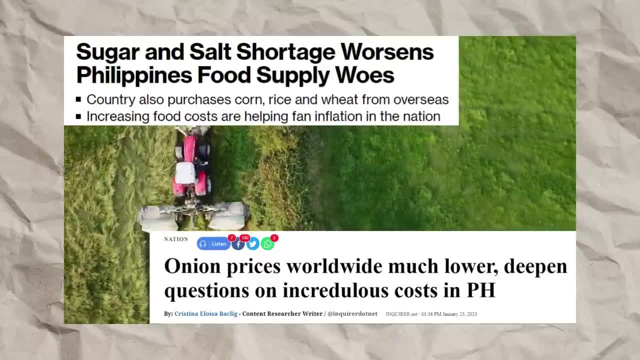 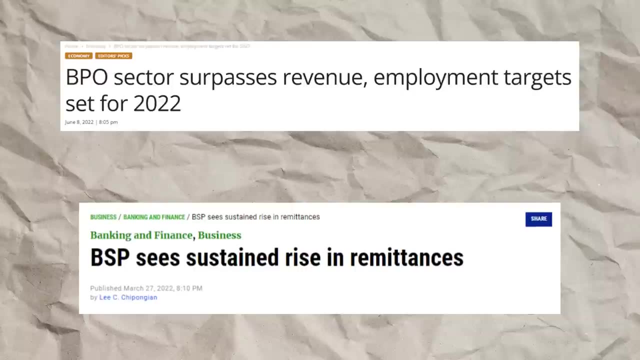 and affected sectors through the extension of reduced tariffs on various products, facilities and an accessible supply chain, among other measures to cushion the impact of inflation on households. But of all of this consistent growth, we must still never forget that along the way, we have seen robust growth in an already strong sector such as the business. 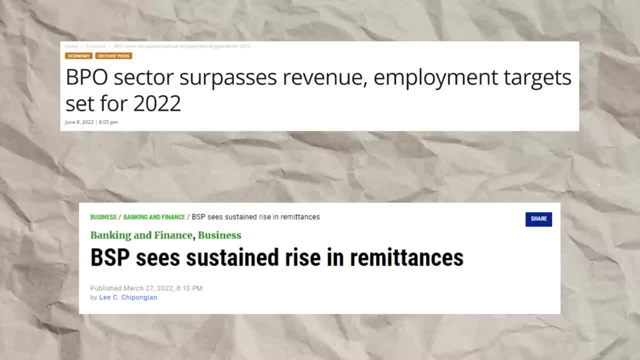 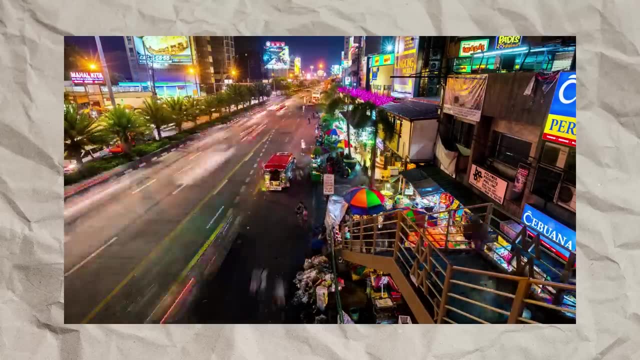 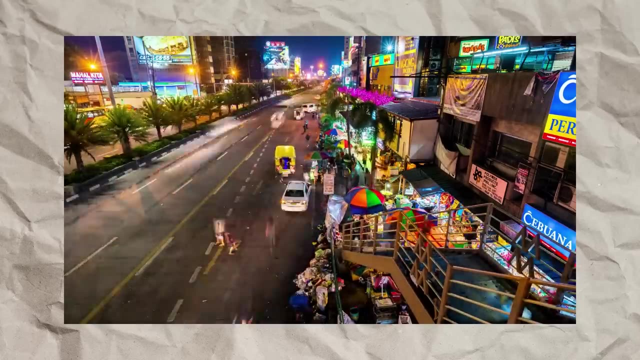 process outsourcing industry, which posted a record-breaking 20% in the last year- billion dollars in revenue, contributing massively to over 1.43 million employees. These were kept in touch and stayed afloat even despite international issues, simply because there were calls to push more for work at home, hence eradicating the need to have 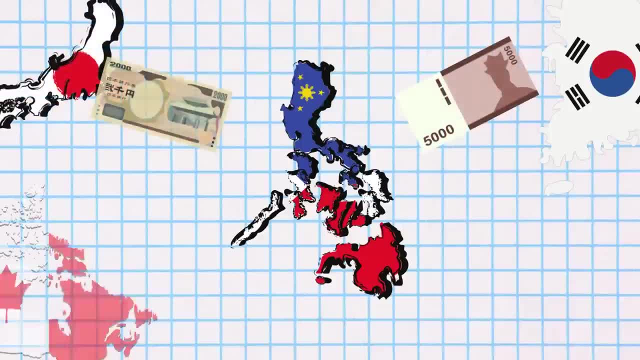 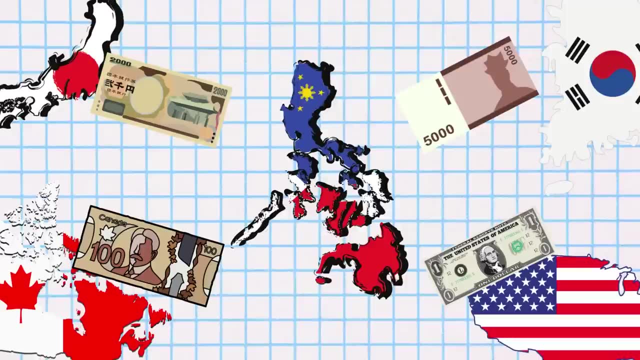 an in-office workplace and more outsourcing. Secondly, we must also praise the strong overseas Filipino remittances, which is estimated to still account for 9.5 percent of the country's GDP. Why does this mean that the country's GDP is still low? 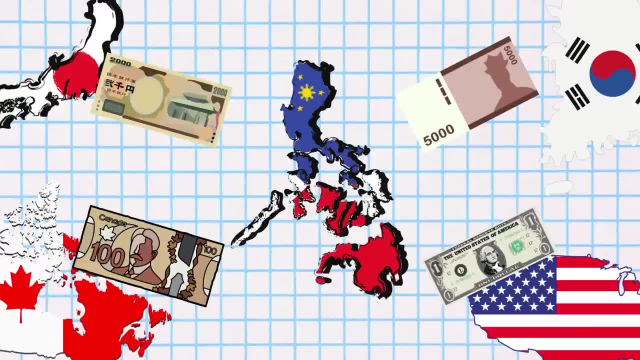 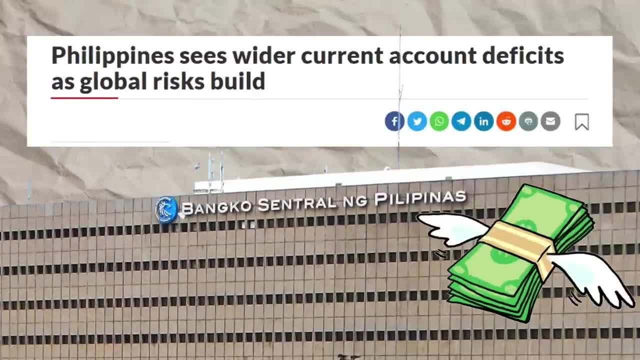 A current account deficit simply means that the Philippines has been importing more goods, services and capital than it exports Without the remittances of about 38 billion US dollars. it is likely that the remittances has helped alleviate the worries about the international 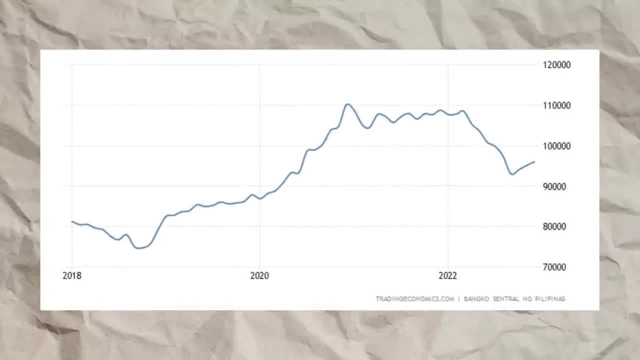 reserve for the Philippines. For further context, the Philippines had declining international reserves in 2022. As of the latest data, it fell to just 96 billion US dollars from around $110 billion just a few months ago. Eradicating, say, the $38 billion received would hamper the foreign. 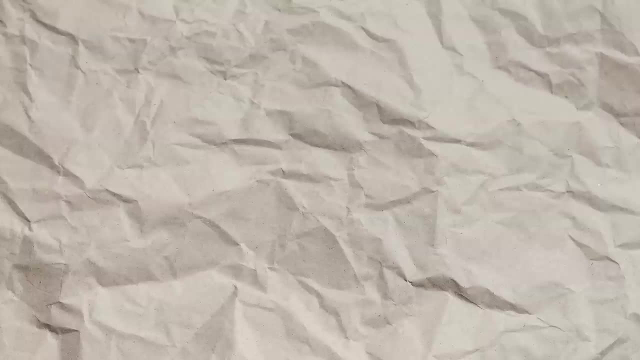 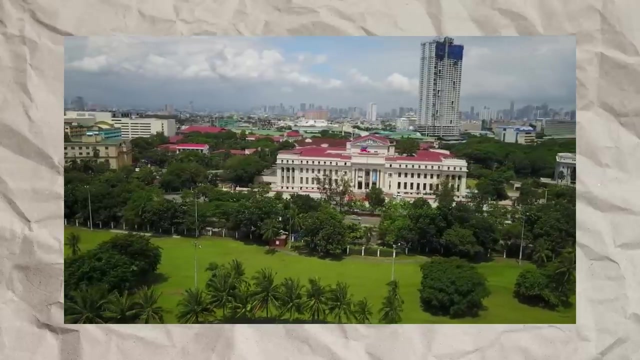 reserves and pose the economy at a bigger risk. Despite this robust growth, there are concerns about the coming year. The country's central bank may need to tighten policy faster in the first half of 2023, which could have an impact on capital formation and GDP growth. 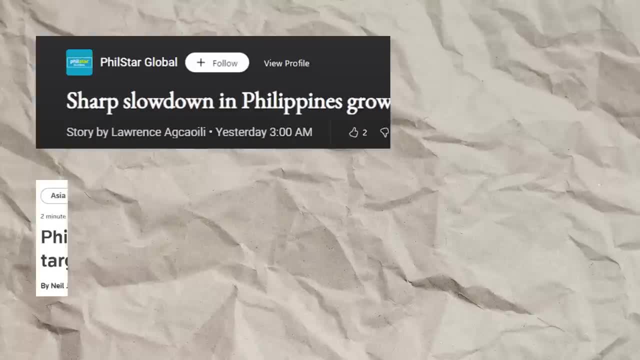 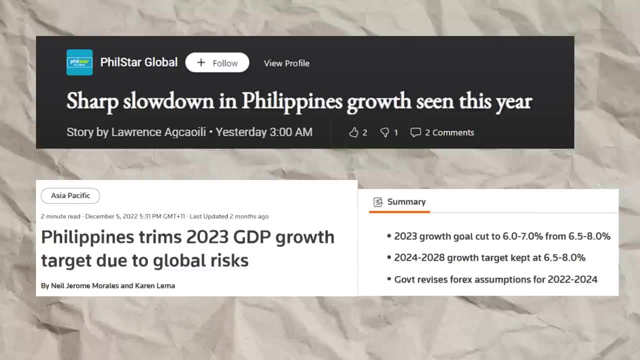 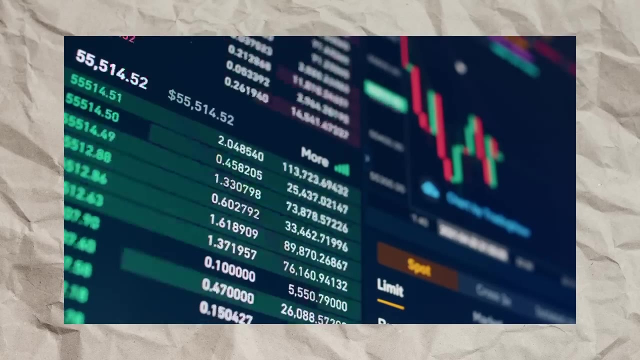 Some official institutions have forecasted growth between 4 to 5 percent, while the government continues to target 6 to 7 percent. However, there is also optimism for 2023,, as energy prices are dropping and the Philippines, being a big energy importer, will likely benefit from this. Some 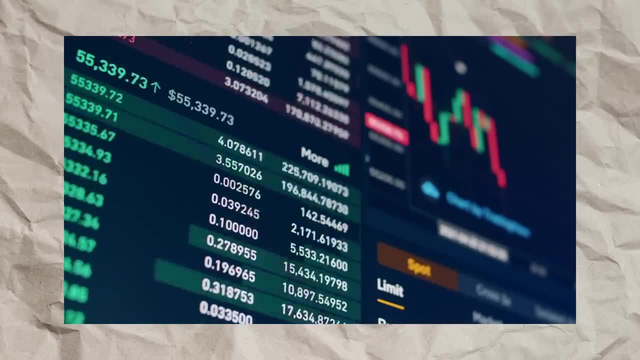 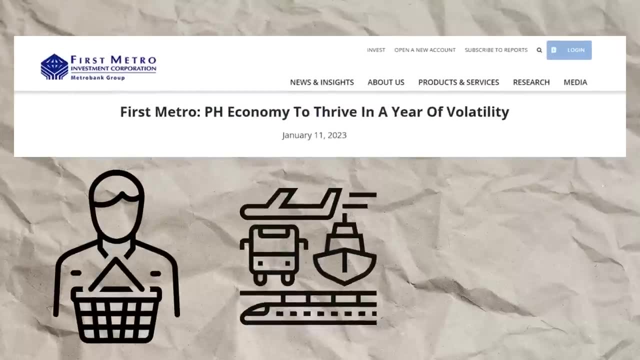 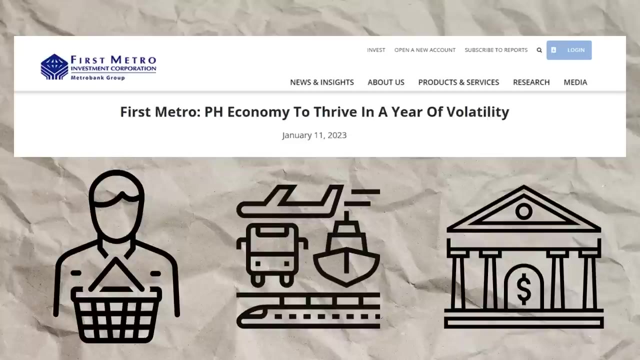 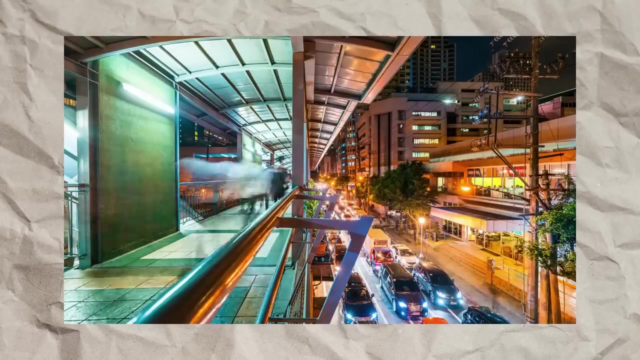 financial groups like First Metro are expecting the Philippines to continue its economic strength in 2023, citing no deep slowdown in consumer spending and optimism in infrastructure. The Philippines' growth in 2022 was driven by a variety of factors, including revenge. 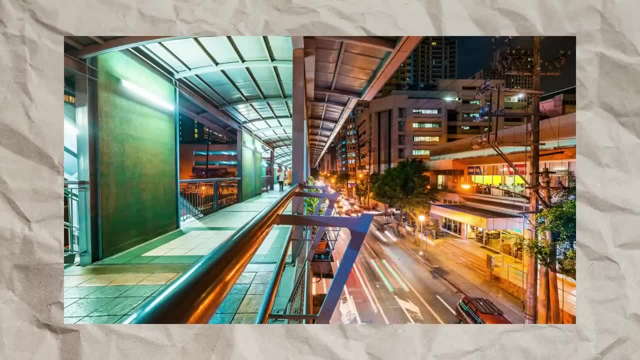 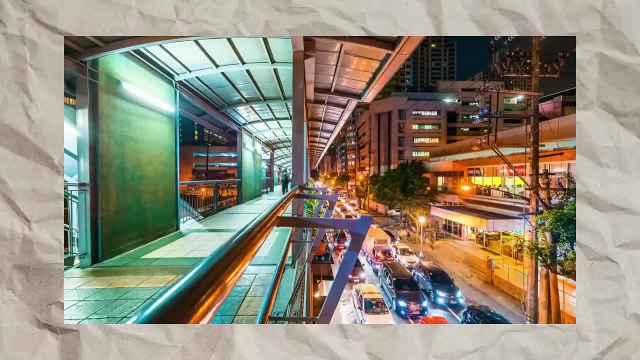 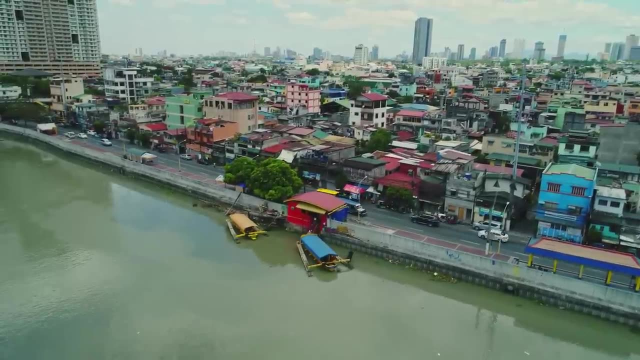 spending, election spending, high employment and a strong performance in industries such as retail, manufacturing and construction. While there are concerns about the coming year, there are also reasons for optimism, as energy prices are dropping and foreign investment policies are expected to contribute to a big foreign investment inflow. Only time 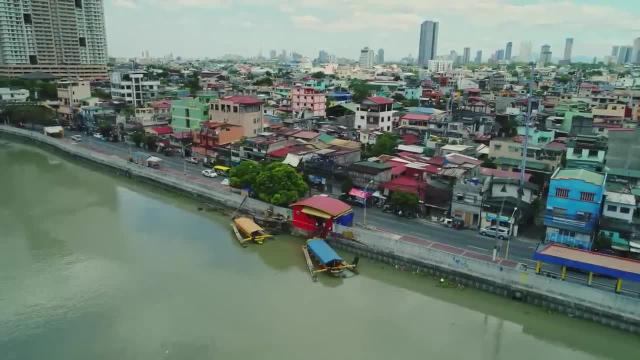 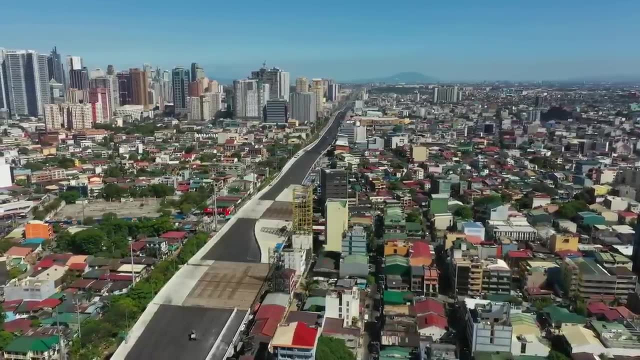 will tell if the Philippines continue to exceed expectations in 2023. But anyway, let us know what you think. What were the industries that shone the best in your opinion? Or even do you think the Philippines will fare better or worse for 2023?? Let us 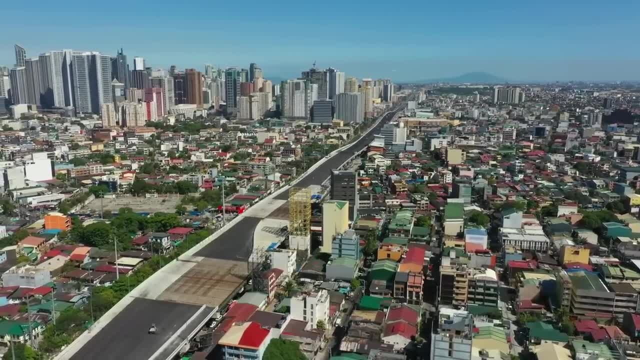 know down below. Thanks for watching. If you enjoyed this video, please like, share and subscribe to our channel. If you have any questions or other problems, please post them in the comments. If you have any questions or other problems, please post them in the comments. Thank you for watching.